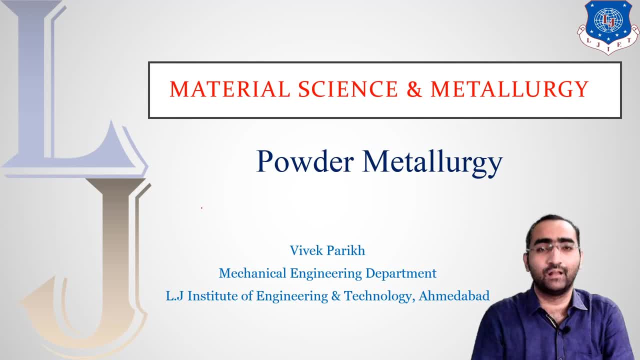 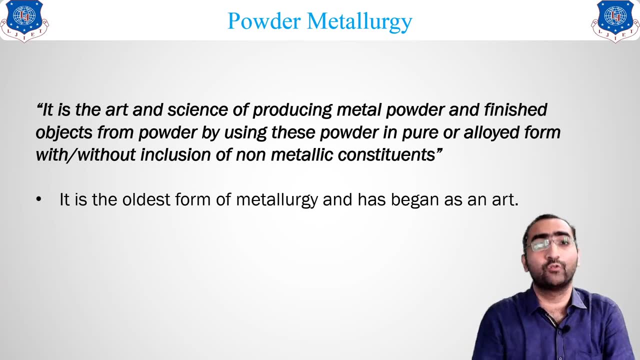 with our next topic, that is known as in powder metallurgy. Now let us begin the thing. that is, what do you mean by the powder metallurgy? Basically, it is the art and science of producing the metal powders and the finished products from it by using that particular powder in. 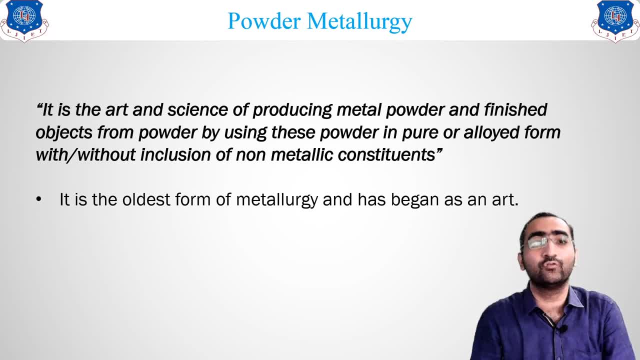 its pure or the alloyed form, with or without the inclusions of the non-metal. That means what we are going to do: we are taking the metal, converting that metal into the powder form and then we are using that powder to make a particularly final product, Now with 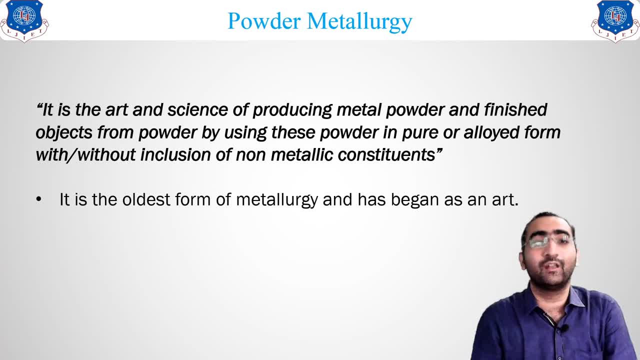 the powder we will be using. we can use the pure or the alloyed. Now we are going to use the alloy powder and with that we can go for the inclusions of the non-metal. that is in our hand. Whether we want to add or we cannot want to add, then it is up to us. 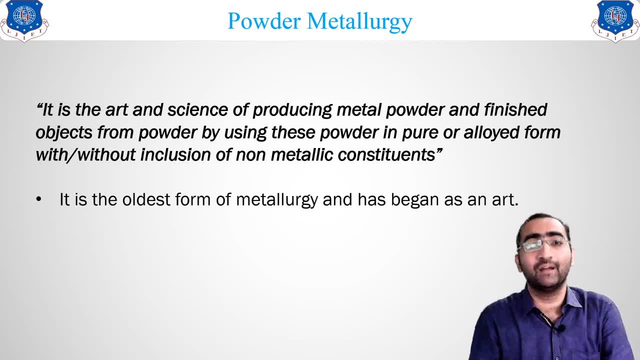 So this is how the powder metallurgy works. That means taking a metal, converting it to the metal, converting that metal into powder and from that powder we are making the final product. so that method is known as in powder metallurgy. Basically it is the oldest form. 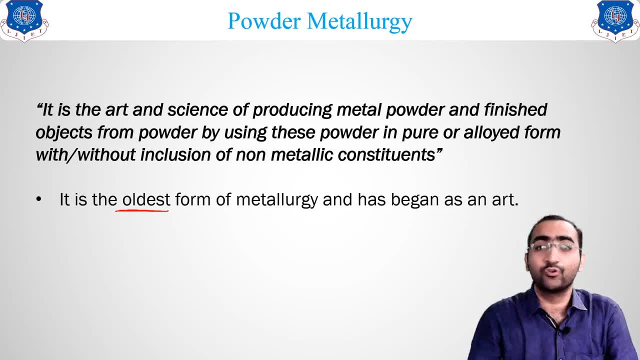 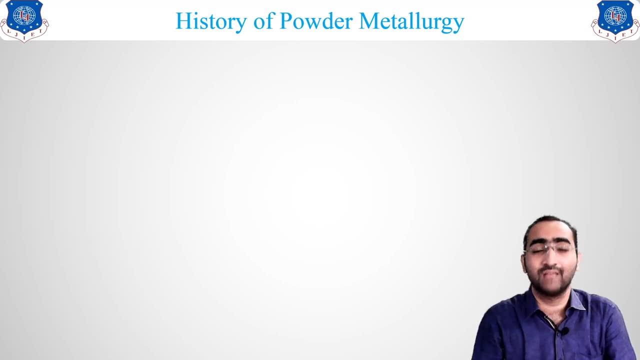 of the metallurgy and has begun as an art. So now we will see that. which are the different evidences through which we can say that this particular method is an older form of the thing? So let us go for the next topic, that is, the history of the powder metallurgy. Now, before 3000 BC, the Egyptian used to make the 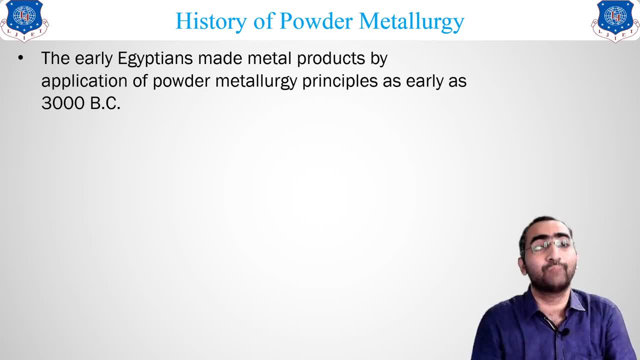 metal products with the help of this metallurgical that is, the powder metallurgy. So this is the basic instinct where we can say that it is one of the oldest form of the metallurgy. Then there is also the history of the powder metallurgy. So let us go for the next topic. 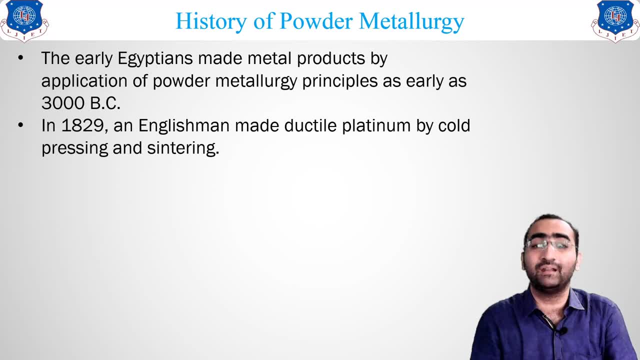 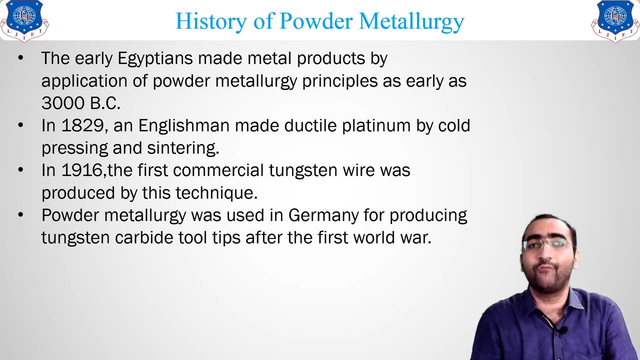 So one of the thing that is. in 1829 the ductile platinum was also made with the help of the particular powder metallurgy. Then comes the tungsten wire were also used by this method. After that the Germans used to make the different types of the material for the war In the World War I. they were used by the help of the powder metallurgy. 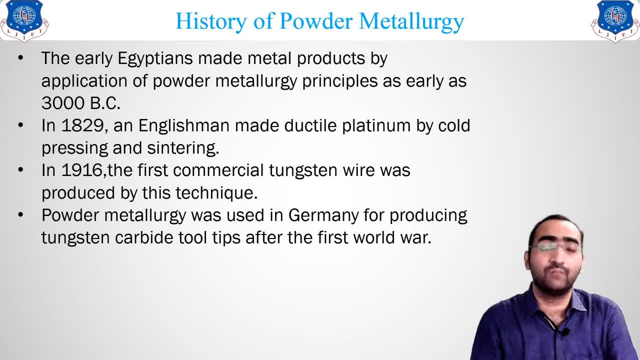 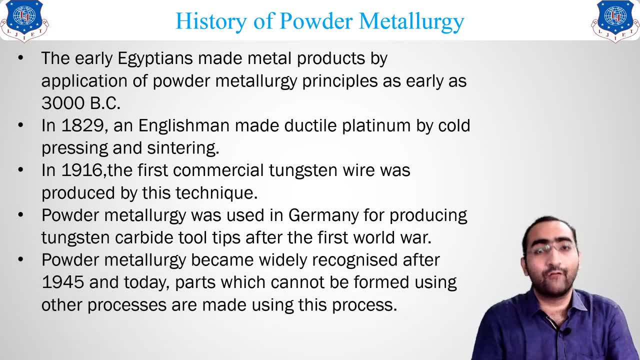 So this is the basic thing where this powder metallurgy come into the existence. That means commercially. if you go, then in 1945 the whole powder metallurgy came into the thing and we can say that it has came in such a way that now a commercial products were used and the manufacturing began at a very rapid rate. 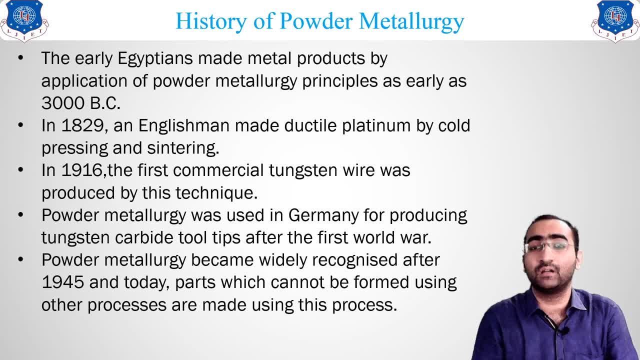 There are certain examples you might be knowing about: the sword of the Tipu Sultan. That is also one of the example of the powder metallurgy. So the researches have also been done Also confirmed that it was made from the powder metallurgy. Then the shields and the cannon balls which were used during the wars between the two kings, and all the shields and the cannon balls were also made from the powder metallurgy. 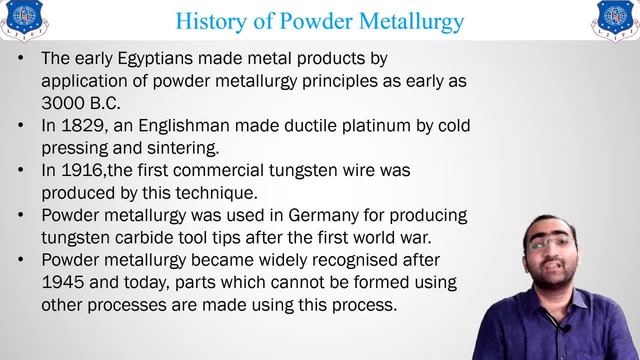 So these are all the evidences from which we can say that it is not one of the modern technology. Yes, there are the different machines which we are using for the powder metallurgy nowadays, But we can say that it has been using. the people are using this particular technology since the many ancient ages. 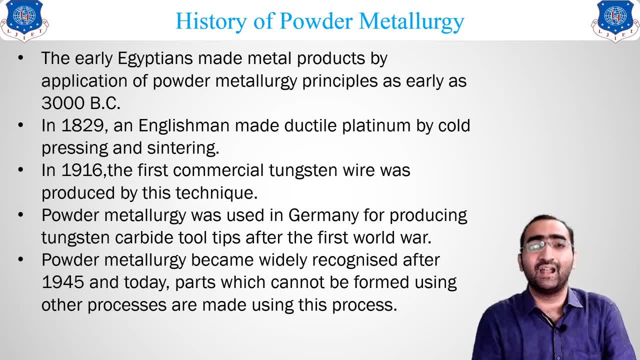 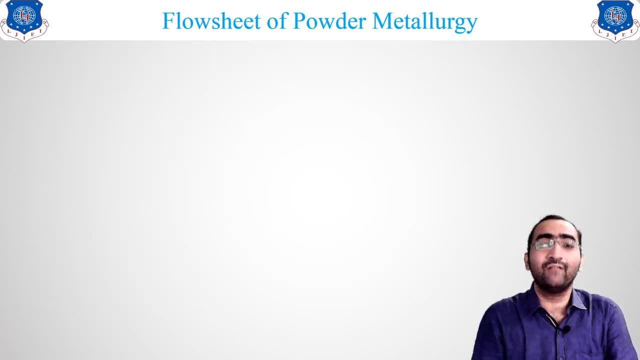 Clear. So this was the history, which suggests that this method is one of the ancient method which is still in the practice Now, where we can see- or now let us discuss about the flow sheets of the powder metallurgy, Now- what the flow sheet of the powder metallurgy looks like. 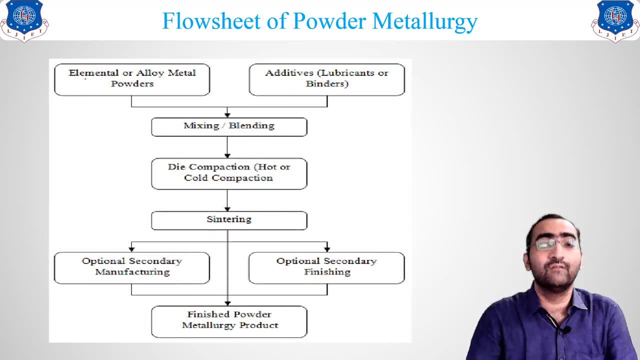 So here it is the thing. What does the first thing we want to take? We will be doing the metals powder, Whatever the alloy. if you are taking an alloy, Then you should be taking more than one One of the metal and then converting both the metal powder separately and then with that we will be using additives, that is, which are the additives, lubricants, binders and all we are using now, both the things we will be adding together and we will be going for the mixing and blending. 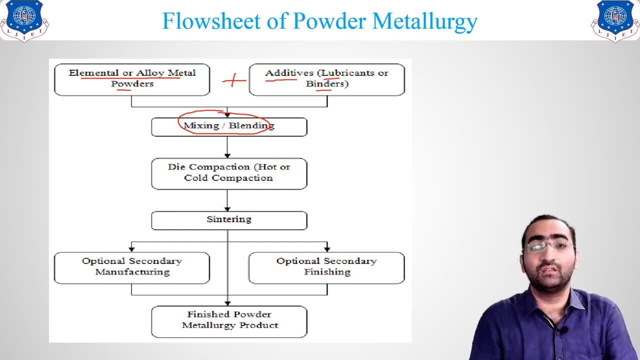 So the metal, metal powder, will never stick with each other for sticking purpose. What we require, we require the additives. So what we are doing, We are adding the additives and the different lubricants. And also what will happen? They will mix with each other. 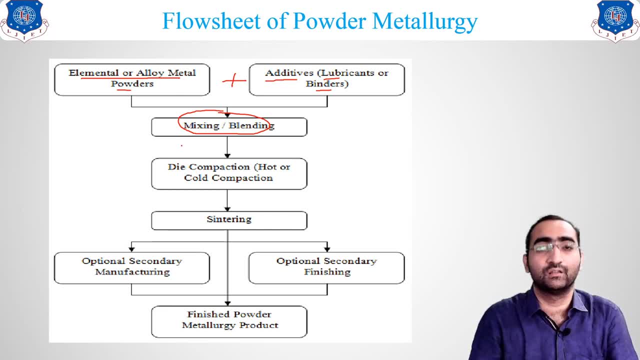 And, as a result, the metal powder will come closer to each other. So that is the mixing and blending. after mixing, what we are doing, We are going for the dye compaction. We are going for the dye compaction. That means we are giving the certain shape to the material. 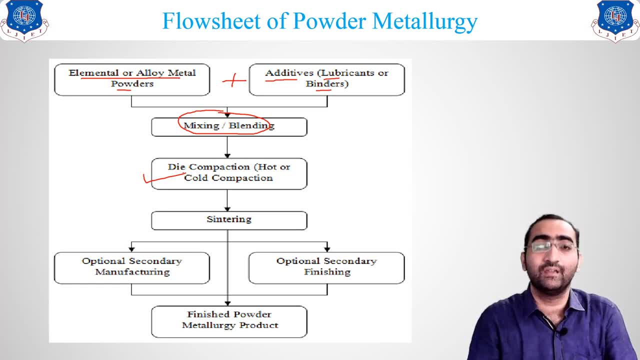 Whatever the final shape we require, we will be giving that particular final shape to the material. So we will. by pressing the material, We will give the final shape of the material. That powder is brought into the final shape. After that sintering is done. 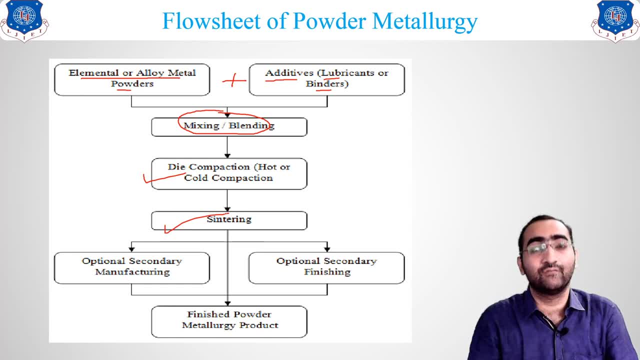 What do you mean by the sintering? Sintering is the thing in which we will be using the sintering. That means we are providing the heat treatment to the material. That means we are heating the material. So what will happen? 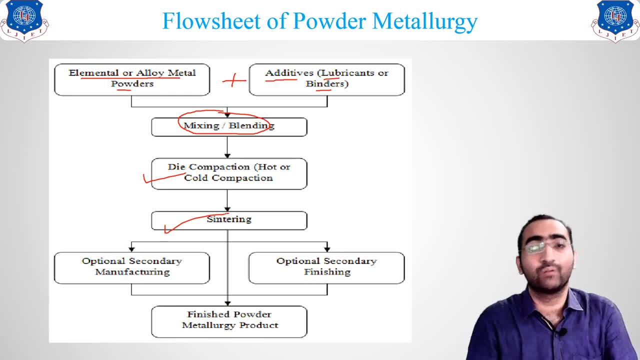 The properties, like strength and all, will increase in this particular thing. After that, that is an optional secondary manufacturing or you can say finishing Secondary, finishing This. both the steps are optional. If you want, you can go as your material is. final product you will be getting. 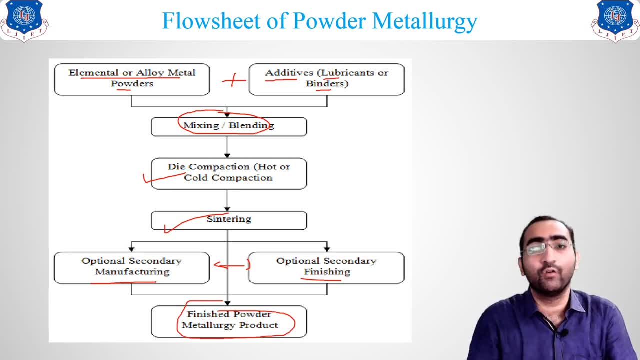 So these are the basic flow sheet, how you will be going or how we will be following for any of the powder metallurgical product. We will be going or we will be following this type of the flow sheet for the powder metallurgy. So now where we are using this particular powder metallurgical product. 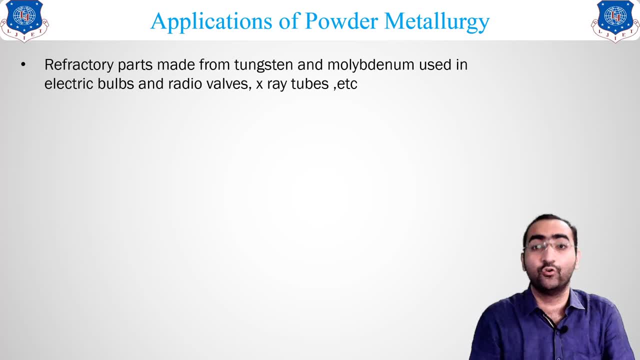 So let us see that thing, that is the tungsten, as I told you, The tungsten rays. that is the filament of the tungsten in the material, The filament of the tungsten in the electric bulb or the radio valve, x-ray tube, all that things, whatever the filament of tungsten we are using, 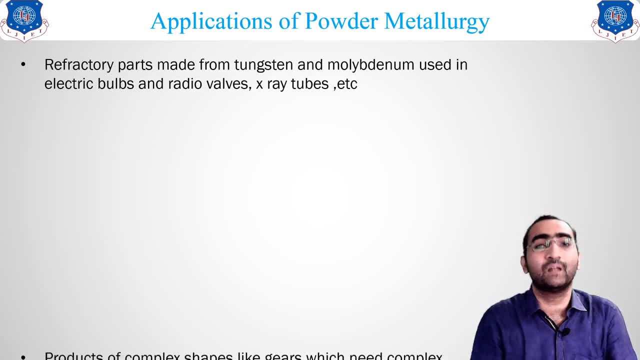 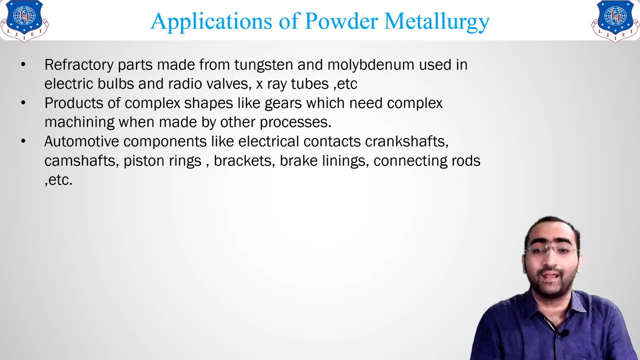 That filament of tungsten is always manufactured with the help of this powder metallurgy. Then the gears and all the complex shape of the gears. they are very much accurately made with the help of this powder metallurgy. Then going for the different types of the automobile parts, such as the electrical contact, crank shaft, piston rings, brackets, brake linings. 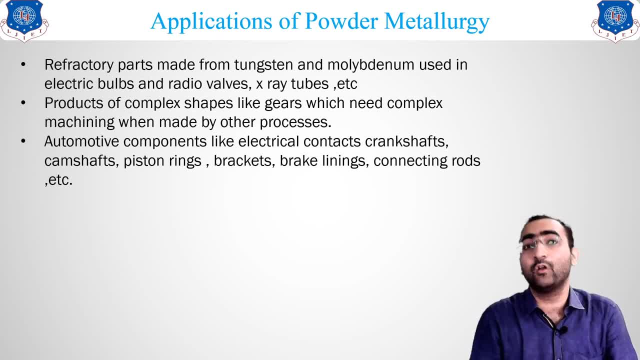 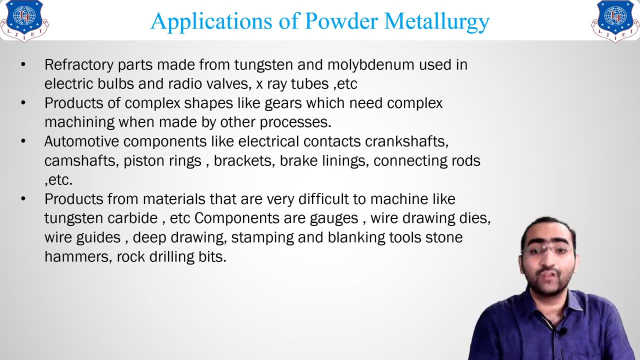 All that thing connecting rock shaft, all that thing. they can also be manufactured with the help of this powder metallurgy. Then the different types of the thing, that is, the things which we are using it for, the wire drawing and all deep drawing. That means the metal shaping, whatever the materials we are using to for the shaping of the material. 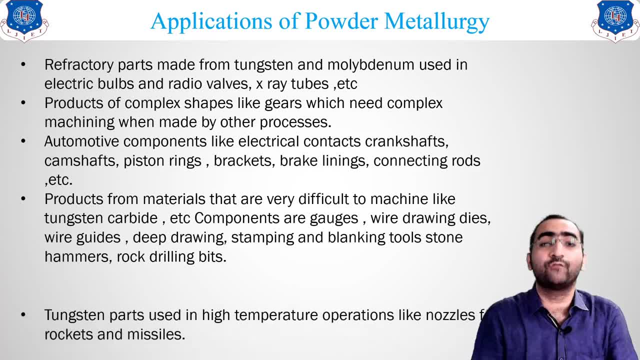 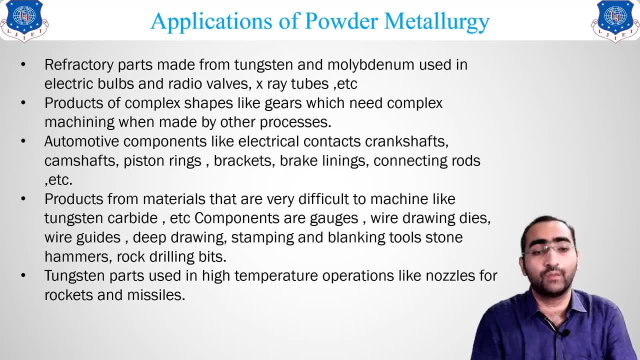 That particular, all the things. they are also made from the powder metallurgy. Then we can say the rocket parts, missile parts and all that things are also made up from the powder metallurgy. Grinding wheel, whatever they are used for, the grinding machining part, clock, timing device, all they are also one of the applications of the powder metallurgy. 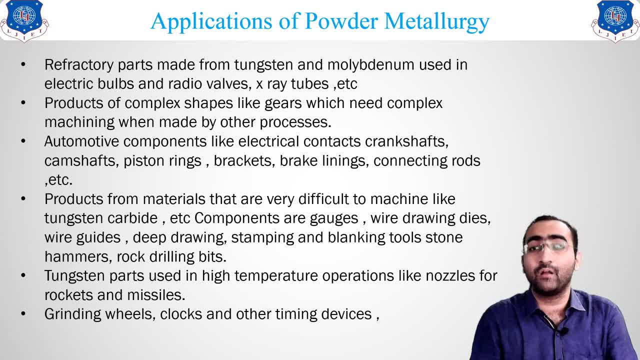 Then the different types of the furnaces also uses the powder metallurgy Lock. whatever the locks- magnets, all that things- they are also made up from the powder metallurgy. That means this powder metallurgy has a very vast applications of the thing. That means it is used in many different fields. 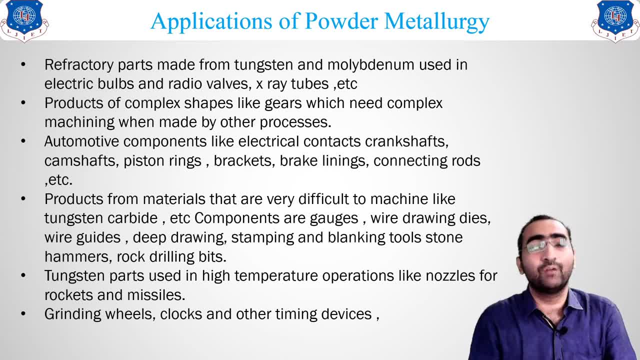 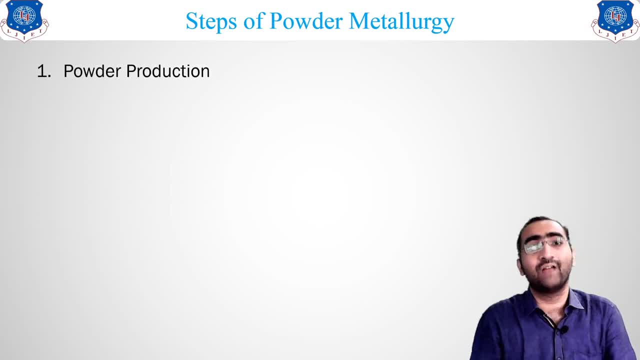 For the many different plants Clear. So for that particular thing we are using this powder metallurgy. Now let us define the steps of the powder metallurgy. The very first step we discussed, that was the very first one we will be going, that is powder production. 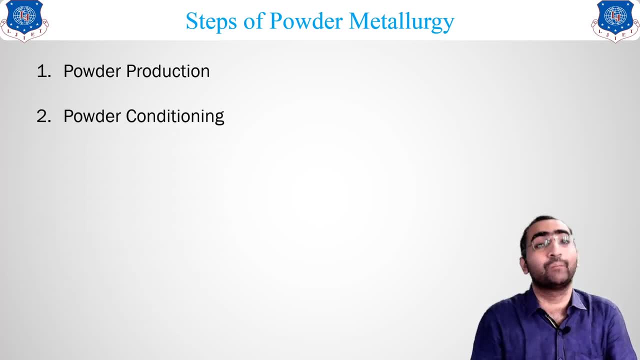 After that we will be following the powder conditioning. The powder conditioning means the mixing and the blending of the material. The third comes the powder compression. Fourth comes the sintering, That is, the heating of the material. Fifth comes the finishing operation. 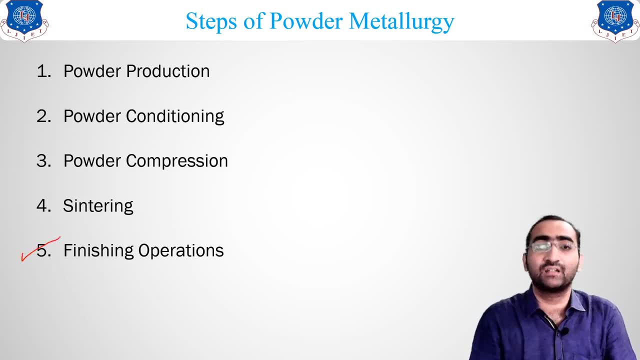 These are the optional, This fifth step that is known as an optional step, and the last one we will be going for the tasting of the material. So basically, the powder metallurgy has been divided into six steps. Out of the six steps, the first four steps- they are the most important and the most widely used step. 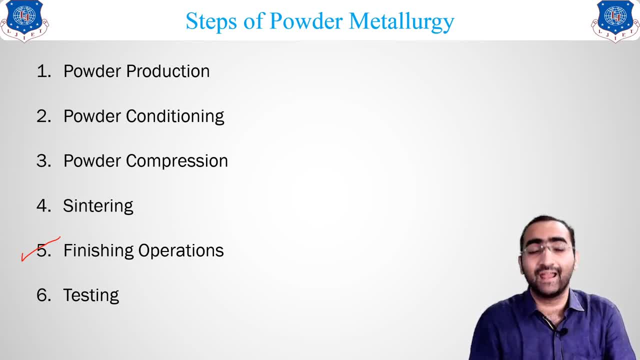 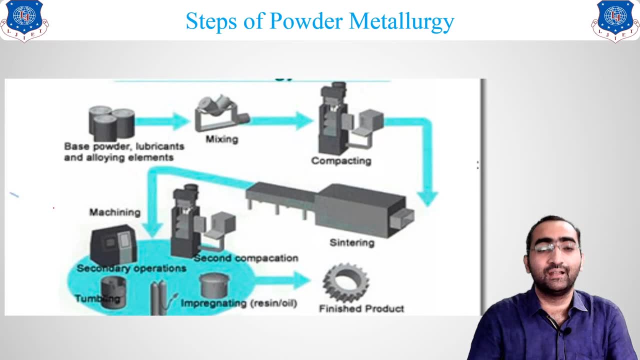 Without the first four steps you cannot manufacture any of the powder metallurgical product, Clear. So now, after that thing, let us see the flow sheet, that is, this is the particular thing, The additives and the powder, which, whatever the material we want, that final product, that thing we are using it over here. 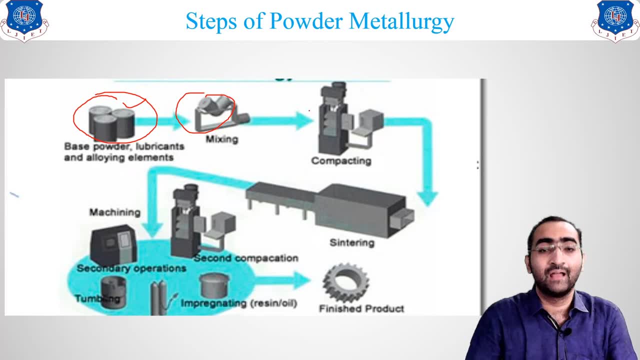 Then, what we are doing. we are going for the mixing part. After mixing, you can see this machine. it will be going for the compression part, So it will compress the material. This is the furnace of the sintering, which the heating of the material will be taking place. 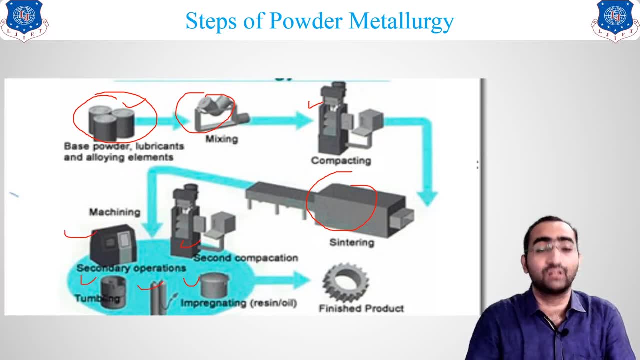 And after that. these are all the secondary operations which we can use And after this operation you can see our final product of a gear. here We are manufacturing with the help of this particular thing. So this is the basic flow sheet of the powder metallurgy and the route we are following for the applications or the manufacturing of the powder metallurgy. 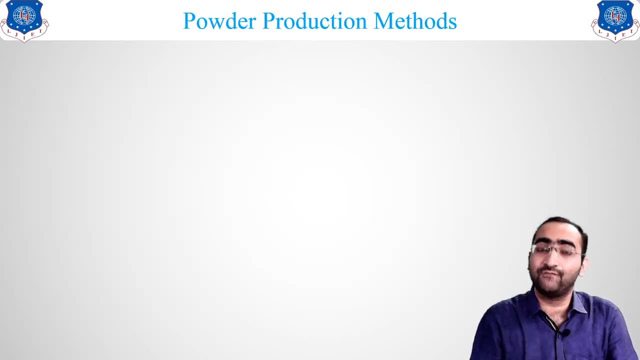 Okay, So now let us start with the very first step. We will be discussing in this whole unit that, the different types of the steps, how we are creating and how we are going for each and every step. So before going to that, the very first step we require, that is known as powder production. 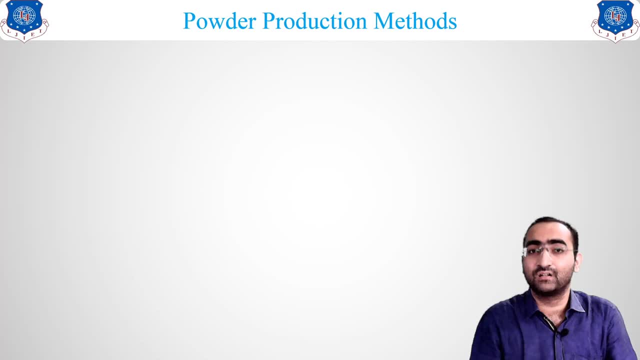 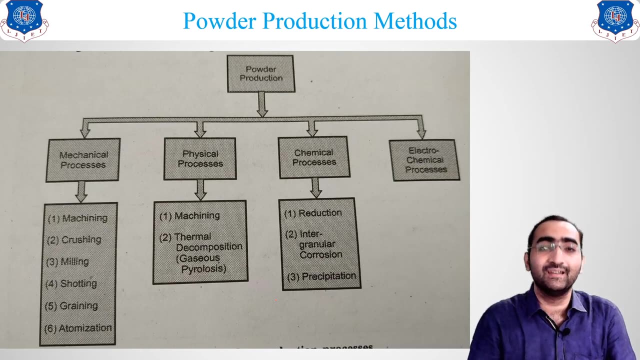 So the very first thing, that the very first step, that is powder production method. So these are all the different methods. All these methods we will be going in a detail in our lecture. So powder production, basically they are divided into four. one, The first one, mechanical processes. 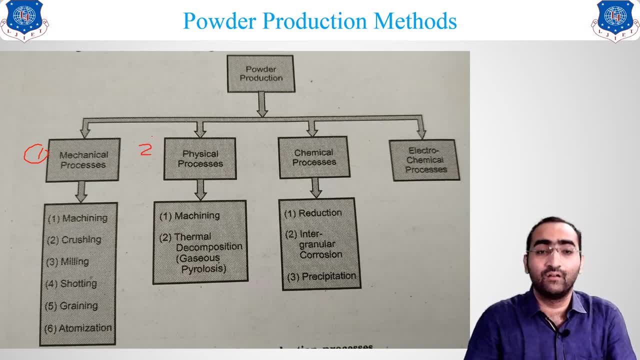 These are the majorly used technique. Second one: physical processes. Third one that is, the chemical processes, And the fourth one that is known as an electrochemical processes. According to the processes, first, the primary classification has been done, that is mechanical, physical, chemical and electrochemical. 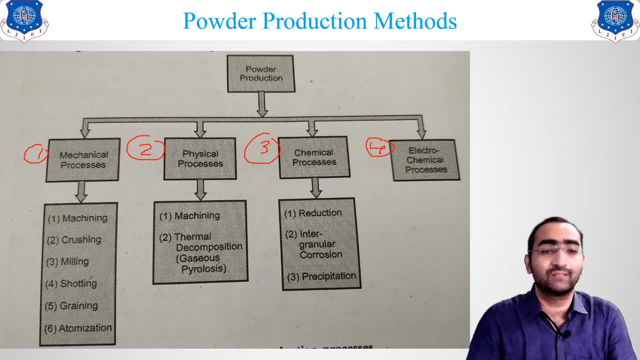 Out of the mechanical processes there are many different six methods: machining, crushing, milling, shooting, graining, atomization And all these things we will be discussing. So in today's lecture we will discuss this- mechanical processes in a detail. Clear. 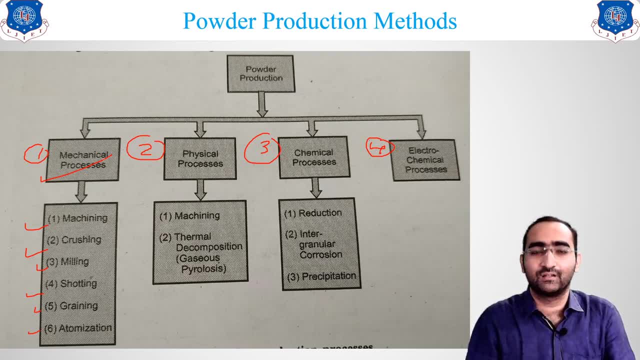 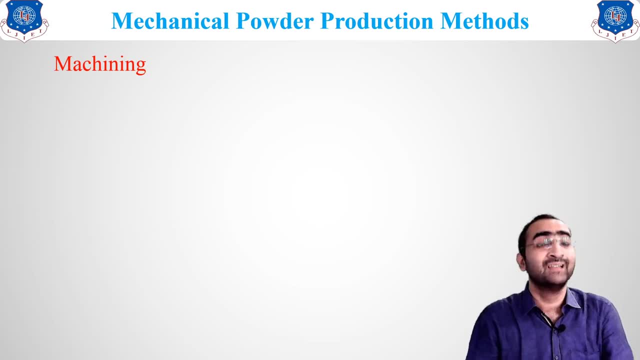 So let us start the different types of the mechanical processes in the detailed version. So starting with the first one, That is, the mechanical powder production method, The very first method which will be coming, That is the most simple method, known as a machining method. 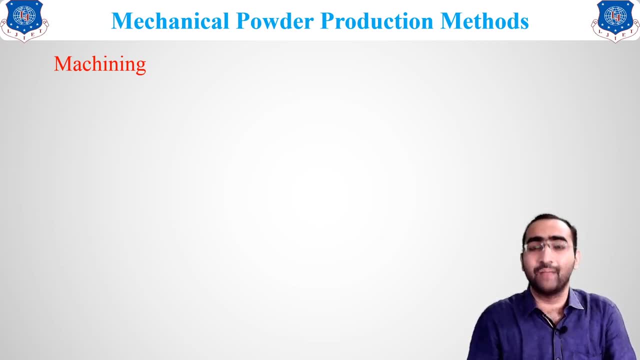 What is this machining method? Machining method is the method in which we are going for the machining of the parts. During the machining, what will happen? The small types of the chips they are formed, Whatever the chips that are getting, The chips we are taking and grinding on the chips. 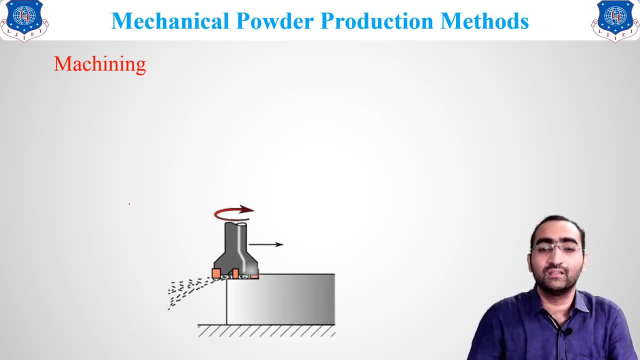 What will happen? You will get the powder. So let us see. See, this is the thing. This is milling, This method. whatever the figure is shown, that is known as a milling operation. During the milling, what is happened? This type of the milling cutter is moved on the surface of the material. 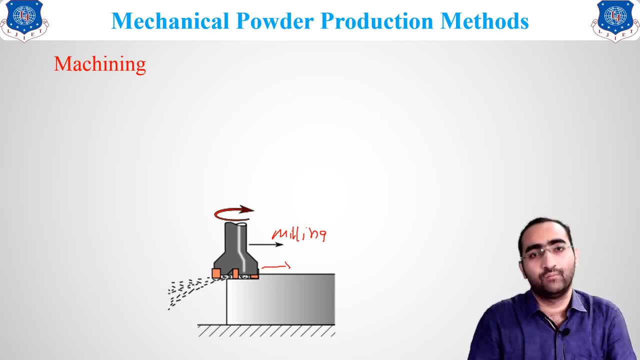 During the movement. what will happen? It will grind the material During the grinding. what will happen? You can see, there is a small types of the chips which are produced. These chips we are taking, They are in a very small form And these chips after grinding or take a particular hammer. 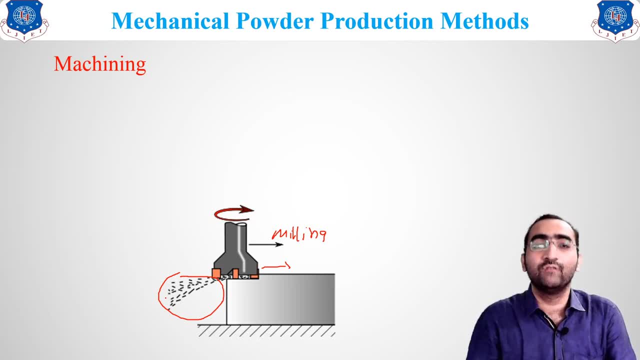 Hit it. So what will you will get? You will get the small particles of the powder, That means the metal we are getting that is in the powder form. So let us see. As the name suggests, method employs use of machine tools to produce powder. 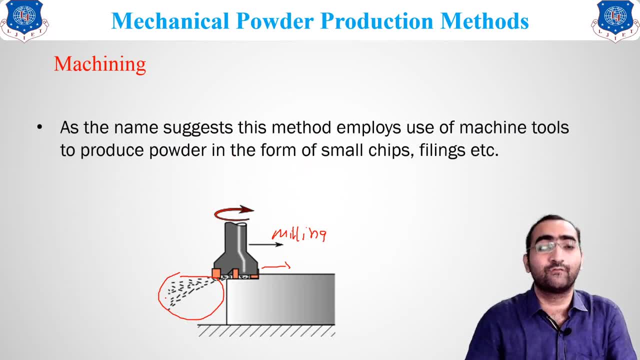 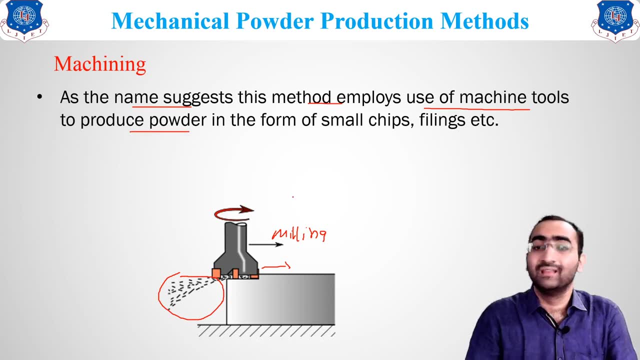 Here I have shown you the thing that is milling. You can go for the drilling lathe, all that machining operation. Whatever, the metal is removed that we can use and that material, by hitting it we can get the powder of the material. The chip obtained are hammered and made in the form of the powder. 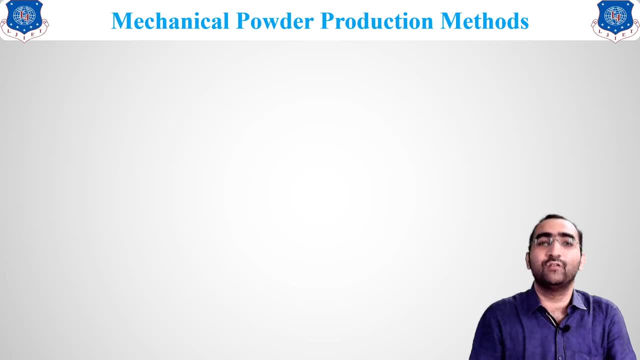 So this was your very first method, which is known as a machining of the material. Okay, by machining method, what we are doing? We are producing the powder. Second method, that is, the crushing, The simple method: crushing. Crushing means to crush the material. 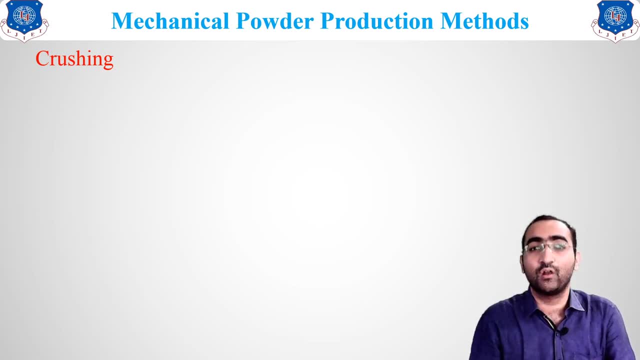 To crush the material, how we will crush Between the two solid part- we are allowing the material to go- and that metal, between the two things, That is the jaw crusher. If one is movable and the second one is stationary, what will happen? This movable will hit the material and, according to it, what will happen? 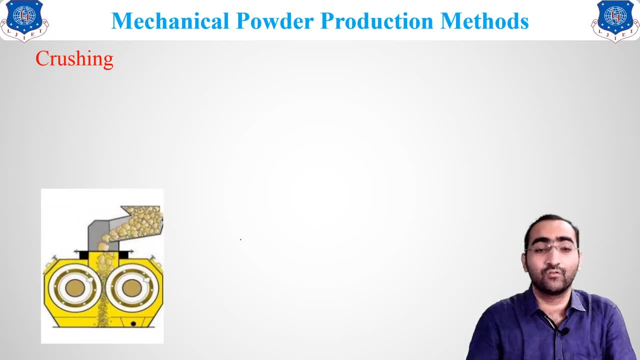 The crushing effect takes place. So here is the thing you can see: This rollers will move, This roller will move and this big particles comes in the small particles, So powder will be getting Here. also, you can see jaw crusher. One is stationary. 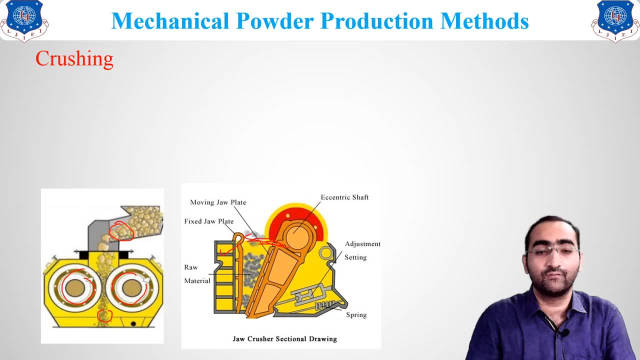 This is stationary part. This is movable. This will move in this way. What will happen During the movement? there is a crushing effect which can be find out from this material and, as a result, the small powders will be coming out from the bottom of the thing. 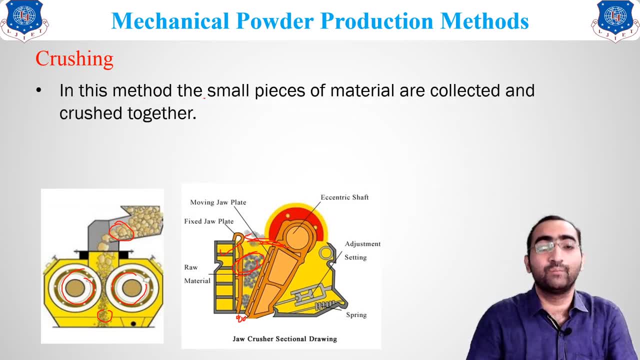 So let us see this method. In this method, the small pieces of material are collected and crushed together. What we are getting? We are getting the small pieces of the material. They are crushed, and what we are getting: We are getting the metal powder at the end. 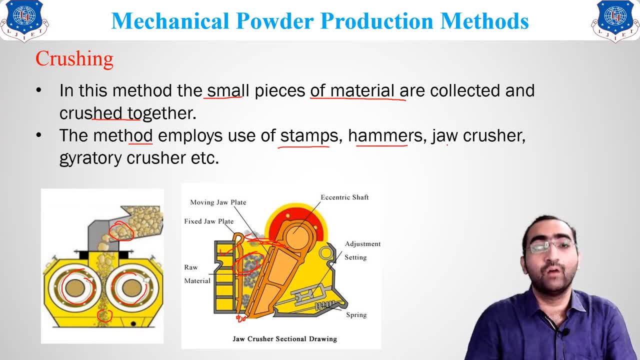 The method employs by using the stems: hammer, jaw crusher, guide rod. So this is the guide rod crusher. Here you can say jaw crusher or the guide rod. By the help of the rotary things we can go. So crushing means basically we are reducing the size of the metal and, as a result, we are 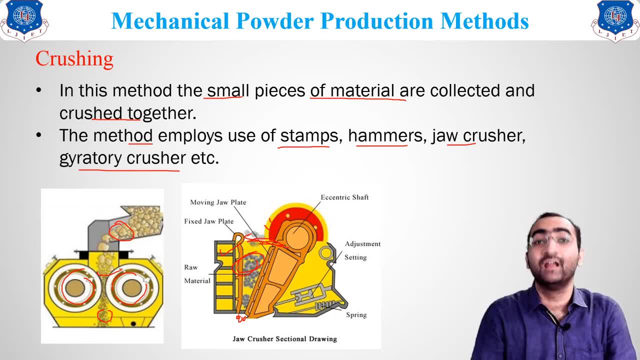 taking so much less amount of size that it looks like the powder of the material. So this is our second mechanical powder production method that is known as a crushing method. Now comes the third method, that is known as a milling method. Now, what do you mean by the word milling? 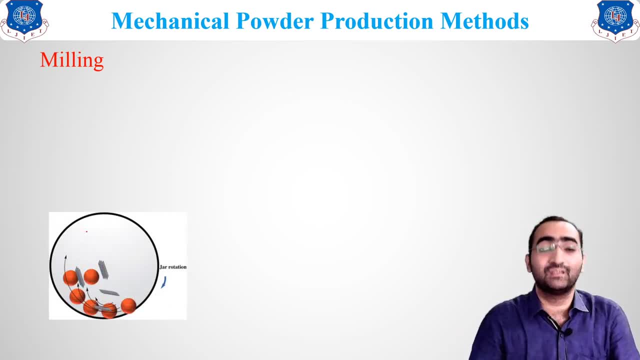 Milling. that is a thing in which there is a one cylindrical drum is taken In that cylindrical drum. what we are taking, We are taking either rod or we are taking balls. Here you can see the balls are taken With that balls, what we are using. 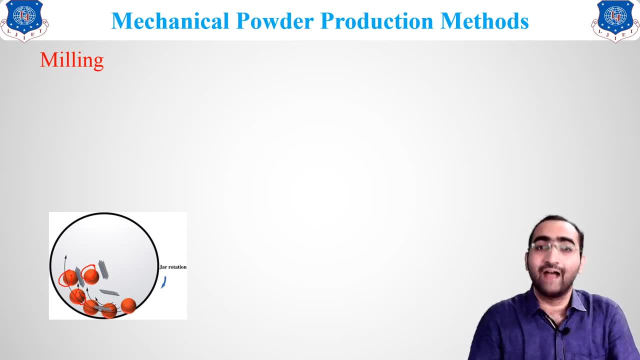 We are taking the metal whose powder we want. After keeping all that thing, this particular mill is rotated. So what will happen? During the rotation? the balls from here will fall down and due to the ball falling down on the metal pieces, it will get heated. 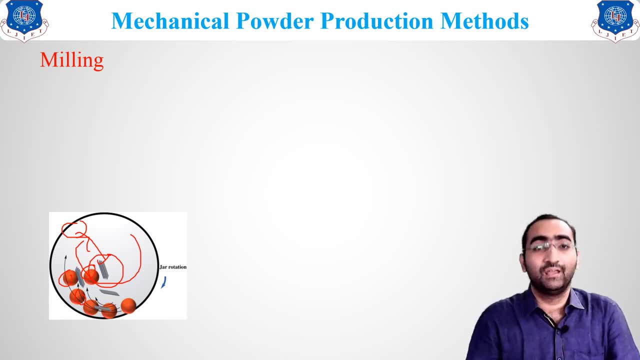 So what will happen? Due to this thing, the crushing effect takes place, So this drum is allowed to continuously roll for a very long time and due to that thing, what will happen? The material will go up and will fall down, go up and fall down, and during that thing, 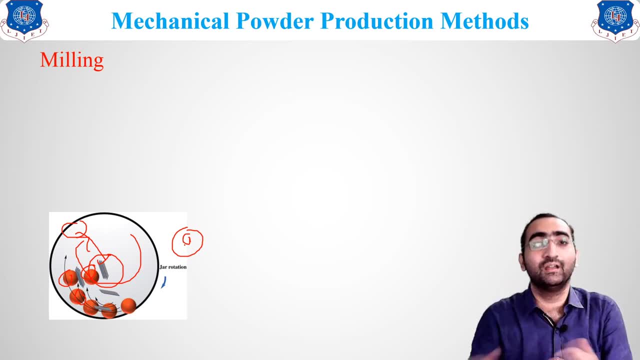 the balls will hit the material and during the heating, what will happen? Crushing effect takes place and, as a result, this thing happens. So this is the cylindrical mill: The balls are taken, Metal pieces are taken and, as a result, this allowed to move for a very long time and due. 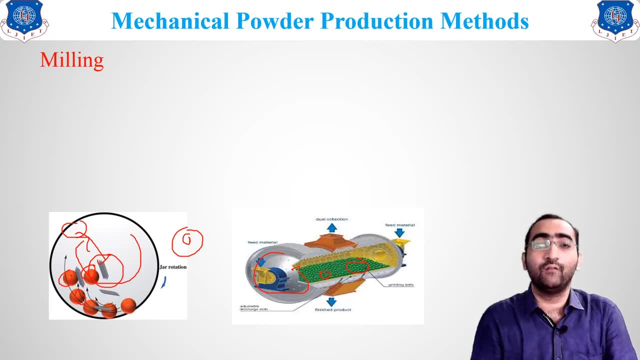 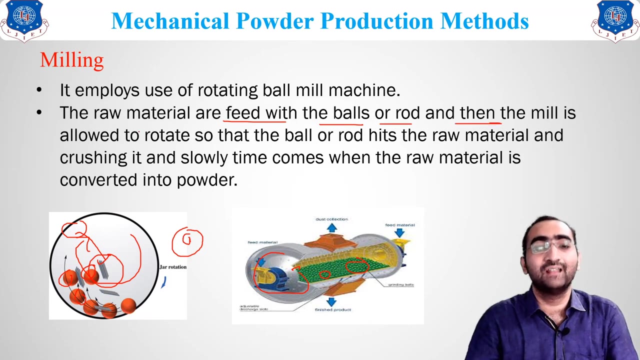 to that thing after a long time. what we will get? We will get a metal which is in a solid form and that will be converted into the powder form. It use of the rotating ball mill machine: The raw materials, they are filled with the balls or the rods and then the mill is allowed. 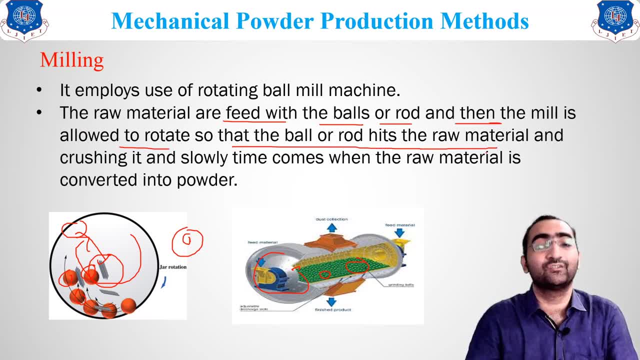 to rotate so that the balls or rod heats raw material and crushing it and slowly time comes when raw material is converted into the powder. So this was your third method, that is known as a milling method. Now comes the fourth one, which is known as a shooting method. 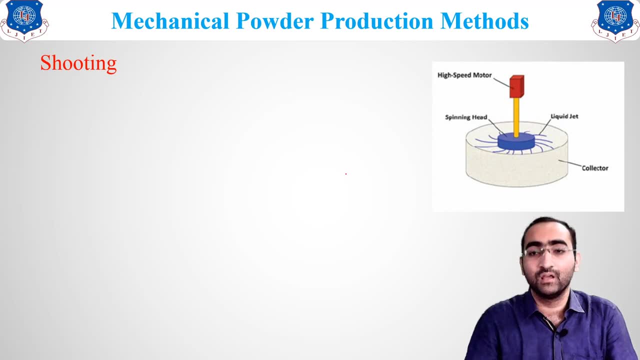 What is this shooting method? There is a rotary thing Here, you can see, there is a rotary table which is moving and on that table, what we are taking, we are allowing a liquid metal to fall on this thing. We are allowing the liquid metal to fall on this thing. 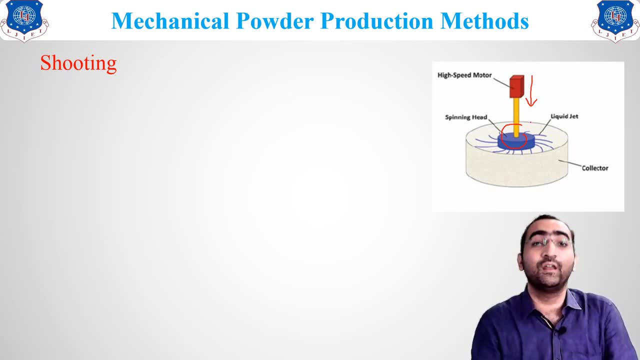 What will happen? When a liquid metal is falling on the rotary thing, the splashes will get away in all the direction. and when this splashes comes down and settle during that during in the air, what happens? the solidification takes place so that liquid droplet will convert into your. 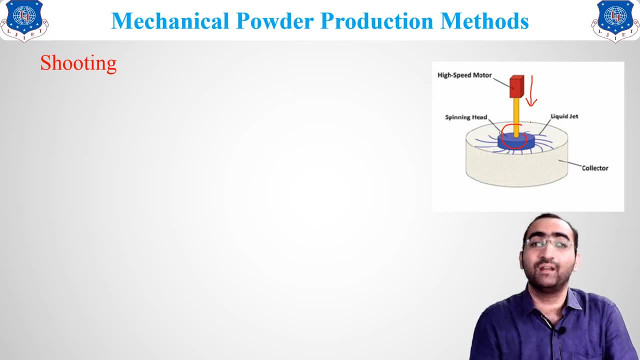 metal powder droplet. That means a droplet is converted into a powder form. So here, due to the help of this rotary motion, what we are doing? We are making a liquid stream into splashes And that splashes are allowing it to cool. and during that cooling, what will happen? 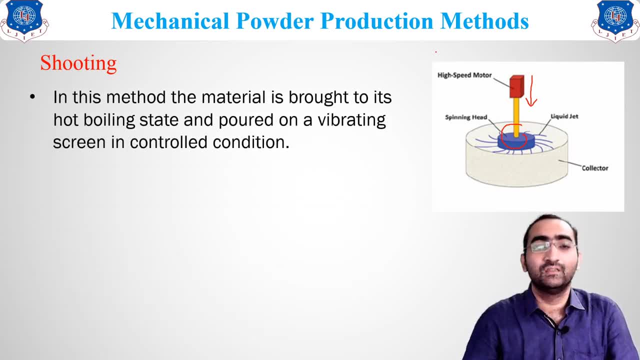 The liquid is converted into the solid. In this method the material is brought to its hot boiling state and then poured on a vibrating screen. in the control condition The liquid droplets are allowed to solidified in the atmosphere. then that process is known as a shooting. 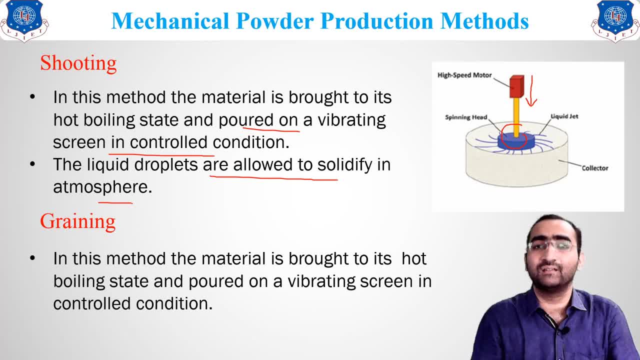 Next method: graining. the method is the whole thing. that is the same. the whole concept is same. So one change: what we are taking, we are taking it. that is the change which we can see. that is, in this graining method, we are cooling it with the help of the water. 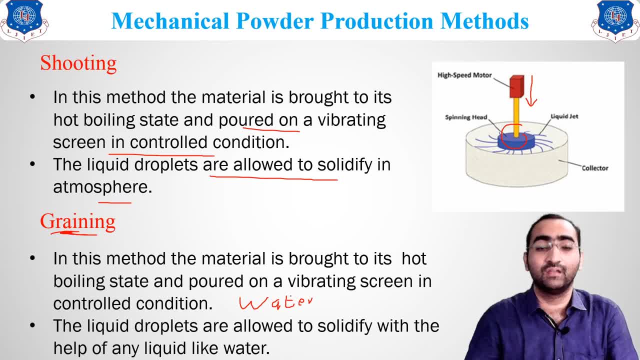 We are cooling in the form of the water or the thing. liquid droplets are allowed to solidified with the liquid, like water. That means the only change that is during this thing. whatever the splashes, they are falling with the help of the water, they are allowed it to cool and as a result of which, 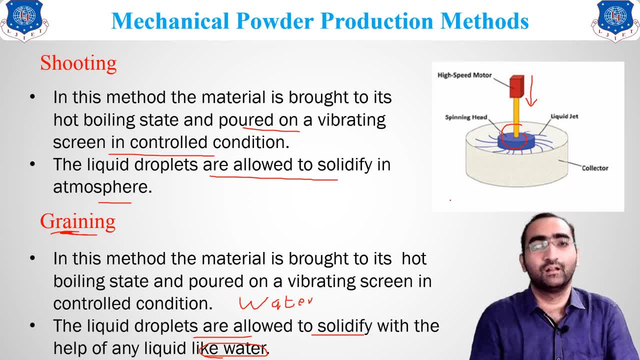 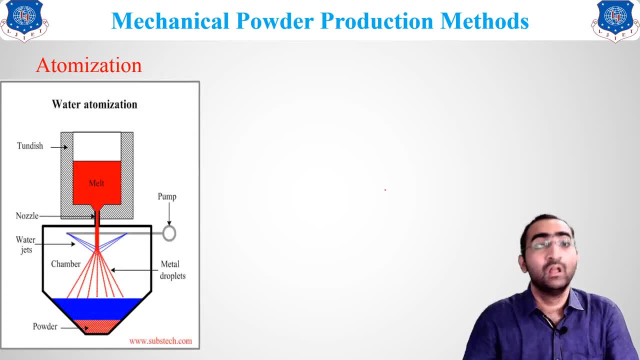 what will happen. You will get the powder of the material clear and the last mechanical method, that is known as an atomization. Now let us see what do you mean by the atomization? the metal is made into the liquid form. You can see the liquid form is taken in the top of the thing: tank. after that it is allowed. 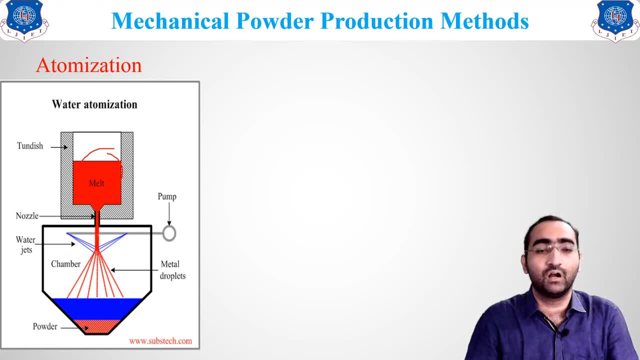 to slowly get down from that nozzle and it will come down. whenever it is coming down, this liquid stream is allowed to cool with the help of the water jet or the liquid, or you can say the compression. So what will happen? during the free fall, that material will get cooled, so this liquid droplets. 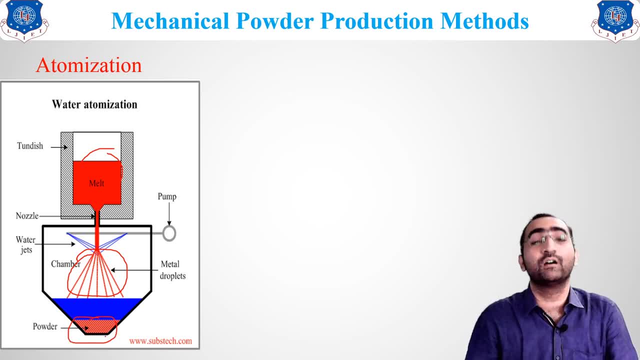 you can see over here, will cool and will get a powder at the bottom of the material. and this method is most widely used nowadays because it is very rapid method and all the material can be easily done powder with the help of this atomization method. Let us discuss the thing. the metal is first melted and taken in the furnace and then passed. 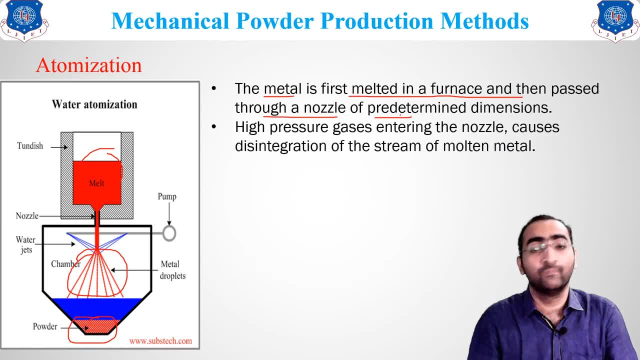 through a nozzle. at a predetermined dimension, High pressure gases, as I told you, enters the nozzle, causes disintegration of the stream. so that means what will happen: due to the high force of the liquid or the gas, the liquid metal will get disturbed and will go at uneven rate with the close control over the metal. 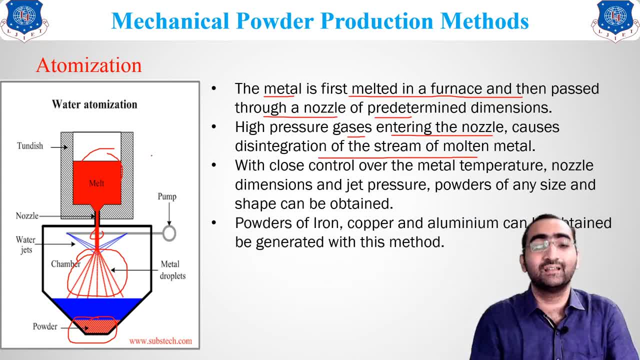 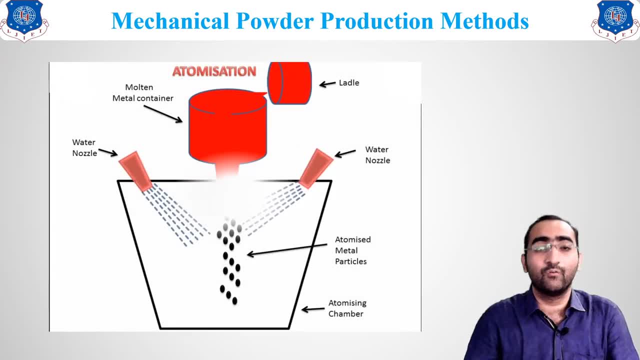 what will happen? it will allow to cool and, as a result, powder of iron, copper, aluminium can be obtained or generated with the help of this method. Let us see one of the one more figure. you can see the ladle we are taking over here. Ladle from that. we are going for the metal container over here. you can see from that. 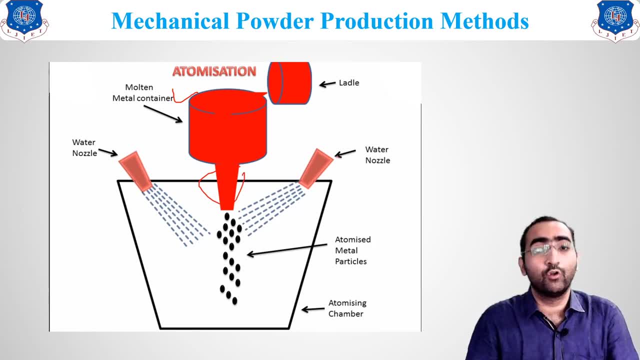 from the nozzle it will come down. what is the role of this water nozzle? it will from the stream, from this stream. what will happen? this stream will be done into the small droplet and these droplets, while coming down, or while falling down, they get solidified and we can. 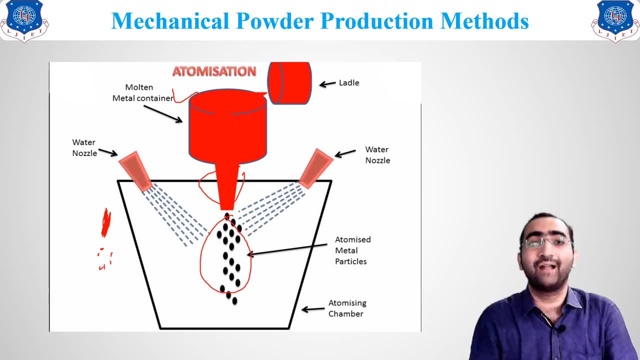 see, that is the small drop of small powder particles. we are getting it, as a result of this, clear. so this was all about the mechanical powder production method and next method of the different powder production we will be discussing in our next lecture. so in today's lecture, what we have discussed. we have discussed the what do you mean by powder metallurgy steps. 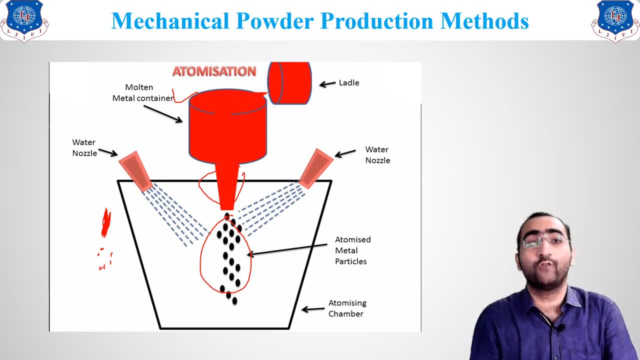 of the powder metallurgy, and then we have gone for the powder production method. that is the very first step, and in that we have discovered all the methods of the mechanical powder production method clear. So this is it, and in the next lecture we will discuss the remaining methods of the powder. production clear till then, thank you.